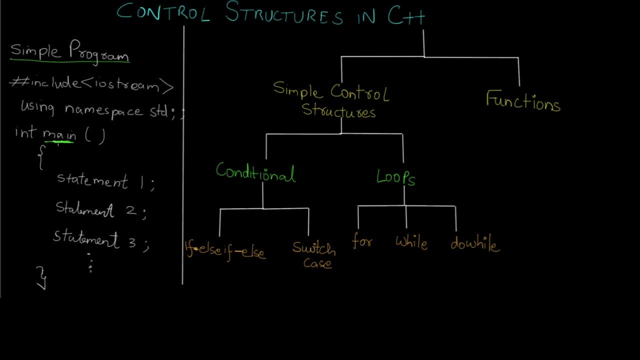 directives. and here you can see the main function is starting. So what happens is, whenever your program executes, basically it executes in a linear and sequential fashion. By this I mean the execution is always in a linear and sequential order. That is it. 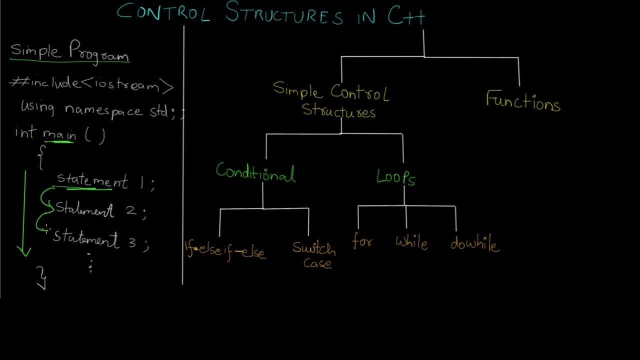 will first execute the first statement, then move to the second, and then move to the third, and so on. But what if you want your program to execute in a different fashion, That is, depending upon statement one and the input or output or whatever the function is happening at the statement one, depending on this value? 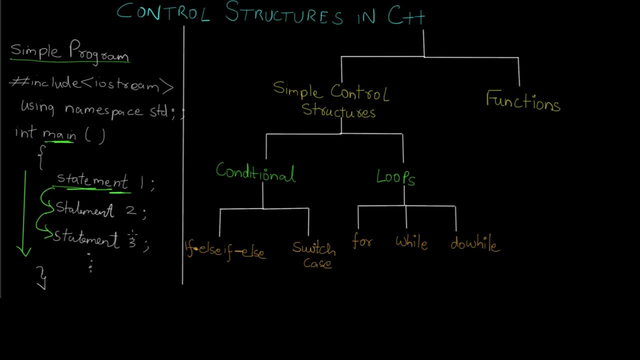 you want either statement two or statement three to be executed. So here is a condition over here, right? So not every statement is going to be executed depending on the condition of statement one. So such functionality is provided by control structures. Another example: 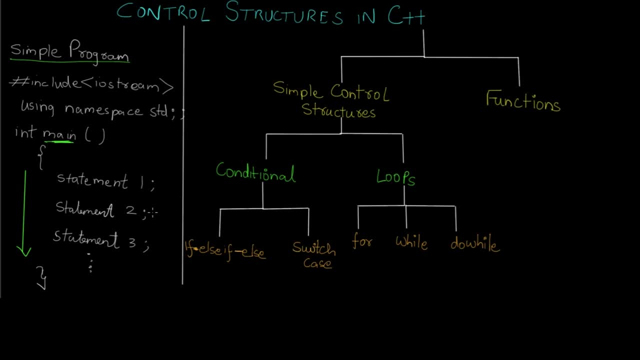 would be what if you want statement two to be executed 10 times? So you will have to write it down 10 times manually. So instead of this, you can use control structures. So these are the two basic benefits of control structures. Now say, for example, you want to perform an addition operation of two variables. 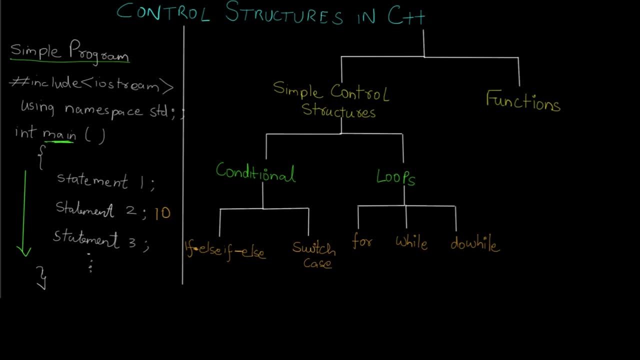 and you are going to be using that for many times throughout the program. So instead of writing the addition operation again and again, you can create what is called as a function in C++ and then use it over and over again. So that will be more beneficial and efficient. 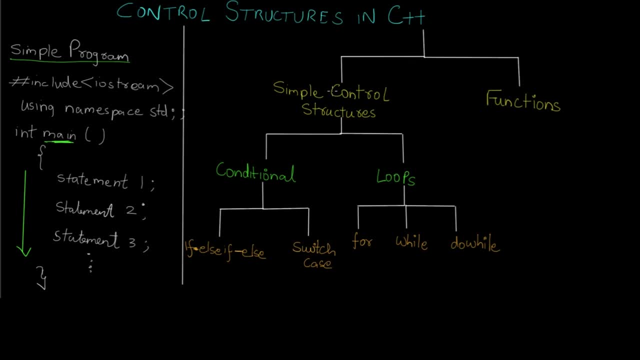 So that is the benefit of control structures in C++. On the right side of the screen you can see I've categorized these control structures into different types. So the first two types are simple control structures and functions. Now, under simple control structures you have 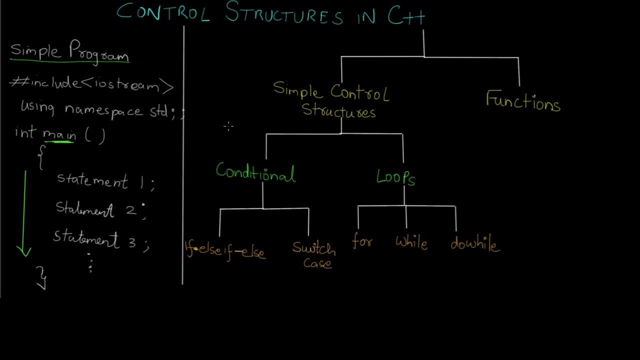 conditional structures and loops. So when you have a condition depending on which the further statement is to be decided or the further execution is to be decided, those type of structures are conditional structures and they include if else, if and else- condition structure And switch case structure. So we'll be seeing these structures in the further tutorials.